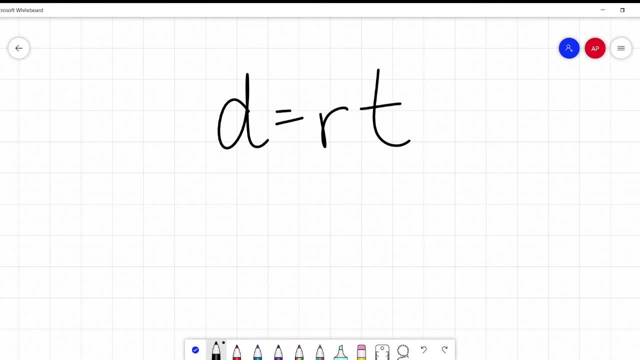 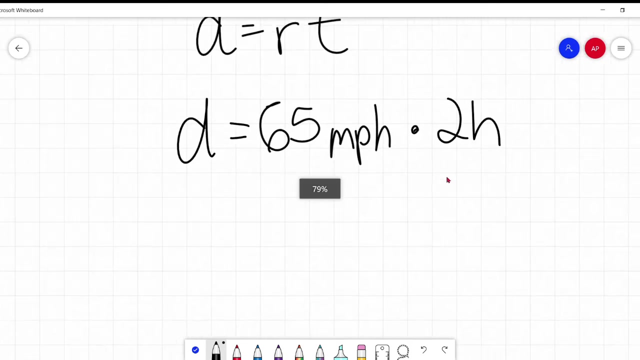 complicated right. Distance equals rate, times, time, And we already kind of know this. If I want to know how far my distance, how far I travel, if I'm going, say, 65 miles per hour in a car and I go for two hours, yeah, okay, 65 times two, That's how many miles? Interesting little. 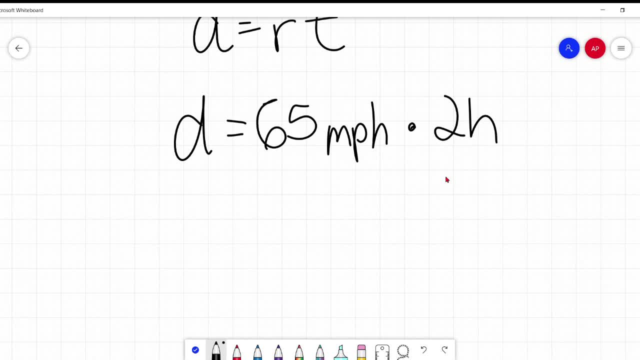 thing here. Well, I think it's interesting. Hope you agree. If not, sorry, you're stuck Just kidding. All right, So miles per hour- you could say miles per hour, That's another way you could write that- And if you're multiplying by hours, those would cancel and you'd be left with 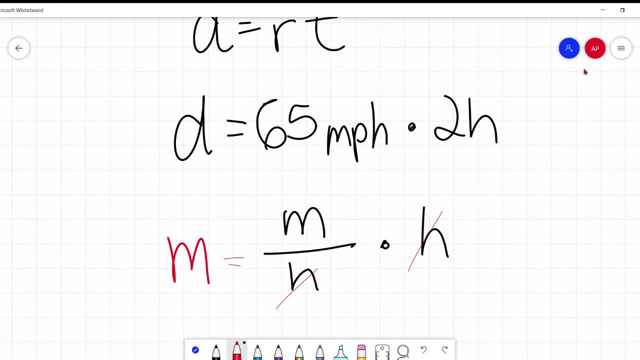 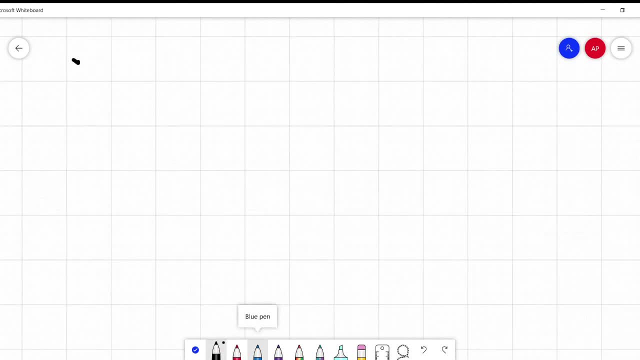 miles. Hey see, it all makes sense. Wasn't that a lovely little detour, All right. So now, distance equals rate times time. That is our overriding one. So here's our first problem. I have two cars that are leaving a central location. They are leaving at 10 am. 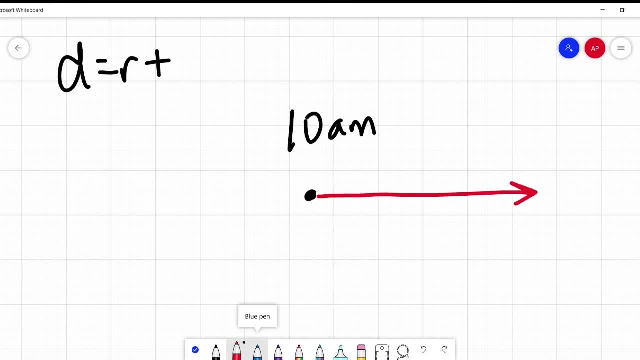 One travels due East, going 50 miles per hour. The other one goes due west. Why are these lines so thin? There we go And they are going. they're crawling along at 30 miles per hour. After how many hours are they 280 miles apart? I'm so trying not to hiccup in your ear. I get the hiccups so. 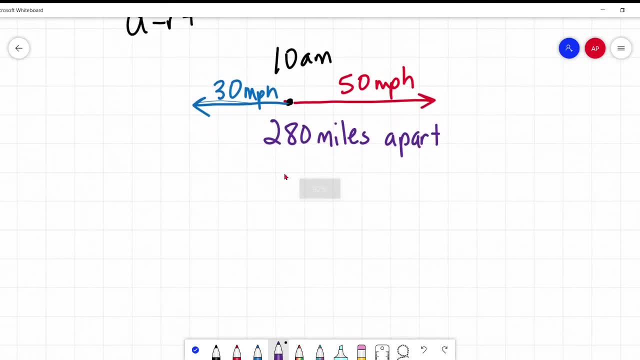 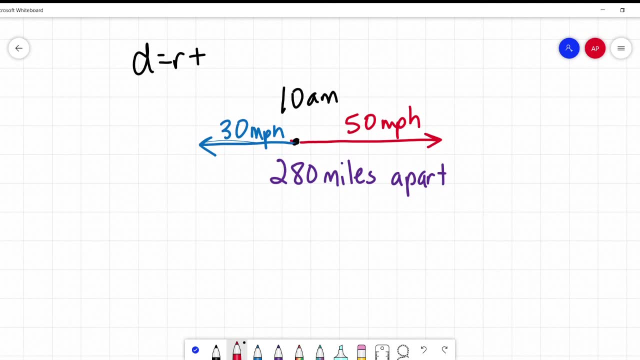 often when I'm talking like this for extended periods of time. I'm sure there is a scientific reason for that, Anyway, OK. So cars: They're driving directly opposite each other on this magically straight road that has no bends and turns, And one. 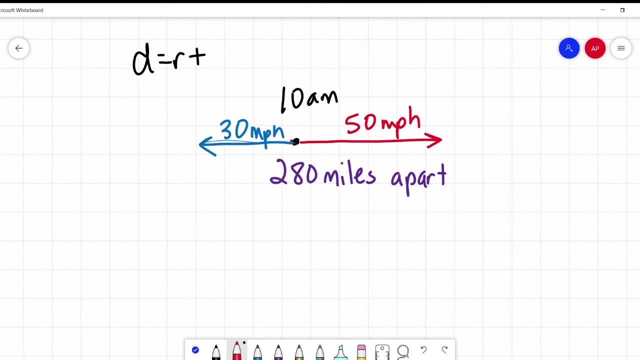 going speed and the other is going like crawling like a snail. So no judgment. if you like to travel 30 miles per hour, you do you. After how long are they? 280 miles apart, All right, So distance equals rate, times, time, A method that I've used that I find works pretty well. to kind, 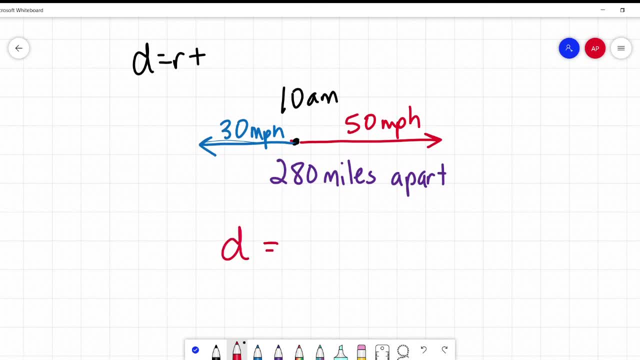 of organize everything is: I do a little, a little chart. I say, okay, distance equals rate, times, time. And then I've got my car, my first car, and I've got my second car. I'm going to fill everything in. So, okay, The distance we don't know. We don't know, um, what portion of this? 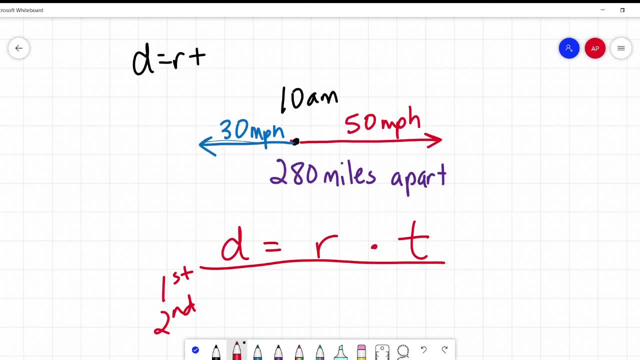 280 miles they each drove. So we're going to leave that alone for now. We're going to fill in what's given, the exact thing that's given in these, and you'll see where we're headed. because you're like, well, the distance is 280 miles, but I don't know what the first car's distance is. It didn't drive. 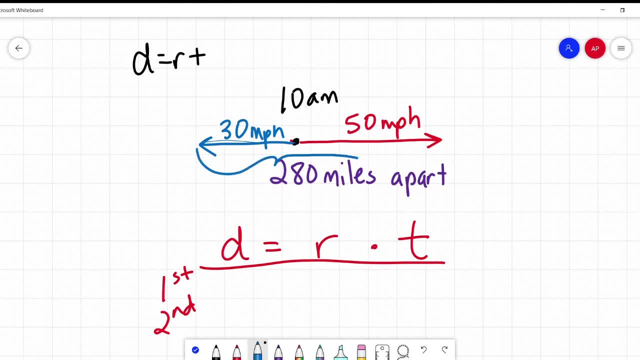 a full 280 miles. Both of them together drove 280 miles, So I don't want to fill that in just yet because I don't know. I don't know what portion each of them drove. We'll get there, Okay. I do know their rates. The first car: 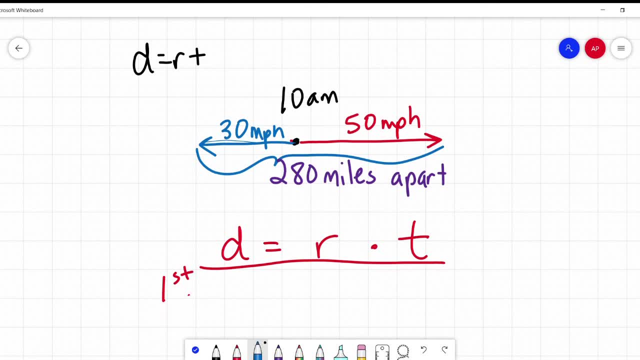 which I'm going to write, and you know what I'm going to write. second in red, So I'm sorry. second in blue, So it'll be really clear which one we're talking about. All right, So the car on the right going East at 50 miles per hour. that is its rate, 50 miles per hour. 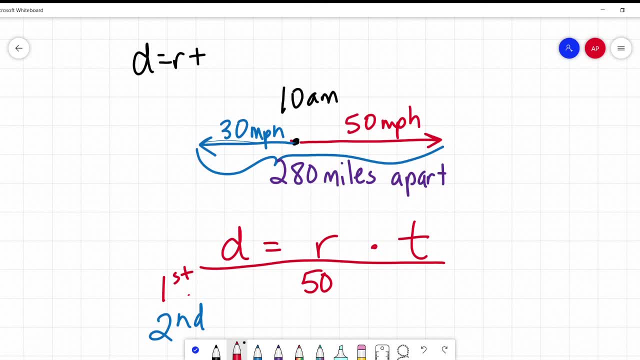 And I'm not writing miles per hour just to keep my little um, keep my little chart clean, but you know that's what I mean. Okay, And my second car, the one going West, is going 30 miles per hour. 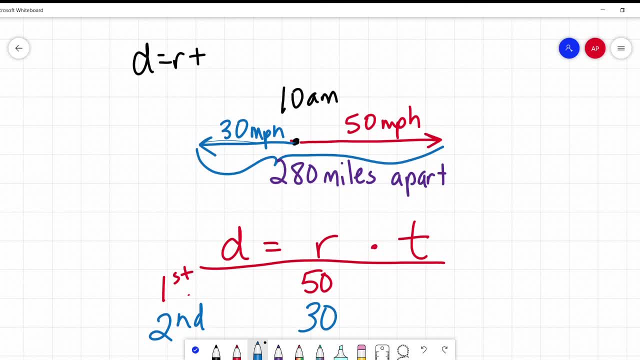 Okay, What is the time? I don't know. I don't know what the time is, So time is going to be our variable that we're trying to find out Now. the time for both of them is the same because they both start at 10 AM and then they don't stop for potty breaks. 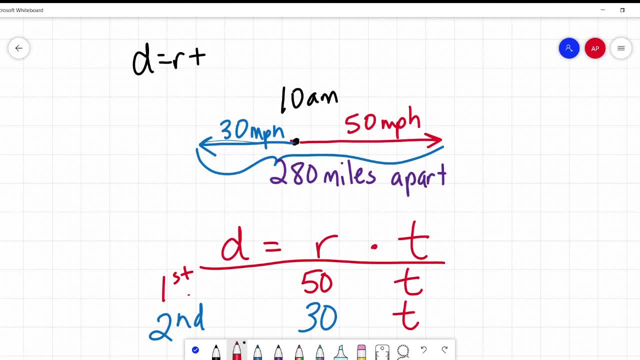 They don't stop at the QT or whatever local gas station you guys have where you live. where I live, It's the QT. So you know they're not stopping at a gas station, They're not stopping for food or you know anything. They're just getting in their cars and driving And then 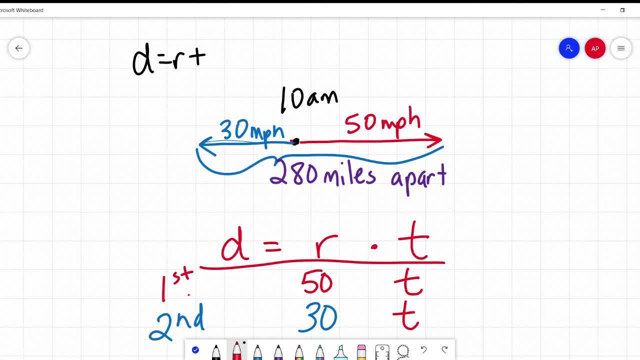 after a certain amount of time, someone calls both of them and says: stop. I'm now calling you to tell you you're 280 miles apart, Cause that's what I do with my life, So that time they've traveled is the same. Well, we know, distance equals rate. 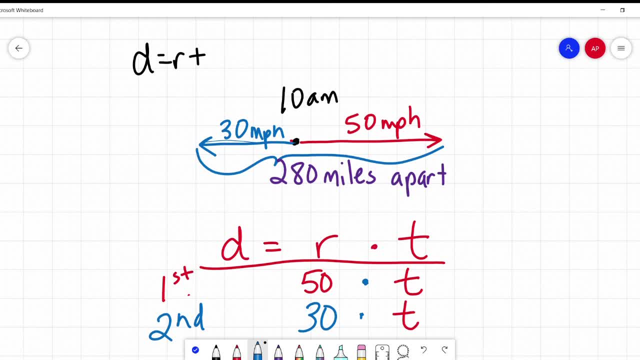 Times time. So that's what I'm going to do. I'm going to multiply these blue. There we go. So rate times time 50 times T is 50 T, 30 times T, And I realized now. I wrote that in red, Sorry. 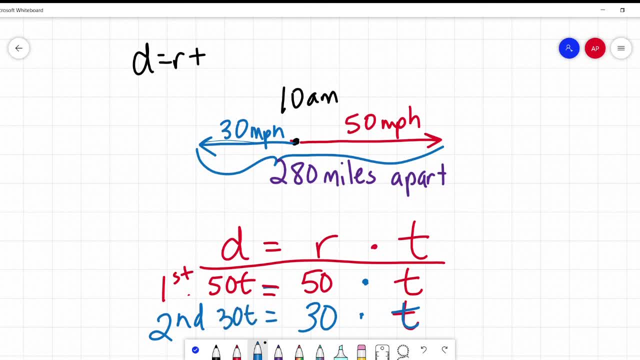 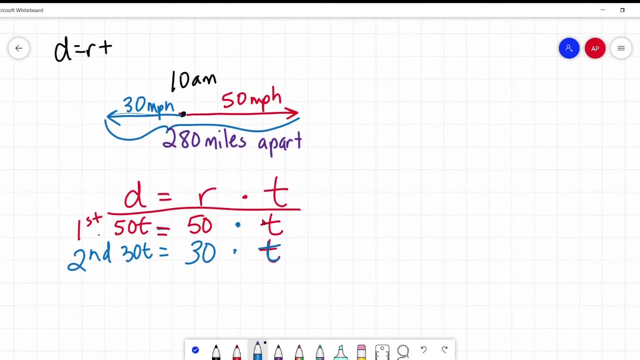 about that. 30 times T is 30 T. So that's their distance. Their distance is 50 T and 30 T. Now altogether their total distance was 280.. So I can say 50 T plus 30 T equals 280.. Now that's. 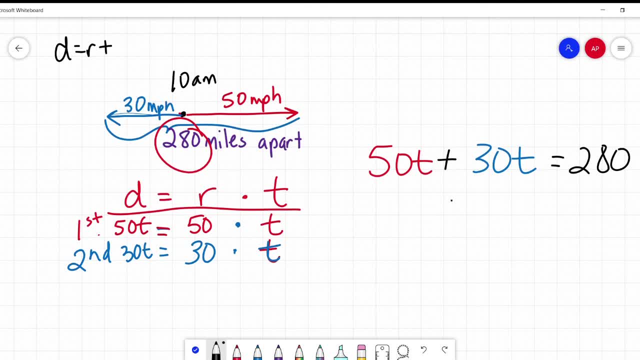 an equation I can solve, and pretty easily too: 50 T plus 30 T is 80 T, And then 80 times T. to that I'm going to divide by 80, and 280 divided by 80 is three and a half. Okay, So three and a half. 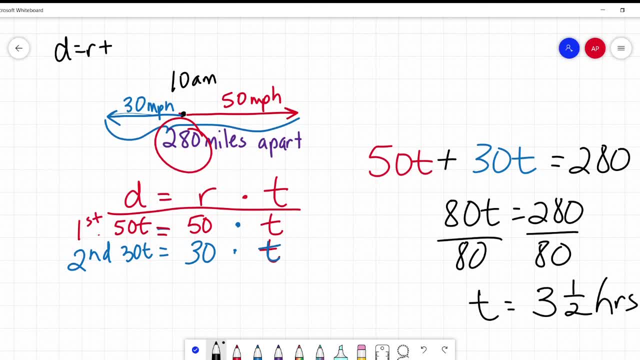 hours. That's how long? Well, so at what time are they? 280 miles apart? Well, it says they start at 10 AM, So I go forward three and a half hours from 10 AM, And don't be afraid to use your fingers to count on this, Honestly. 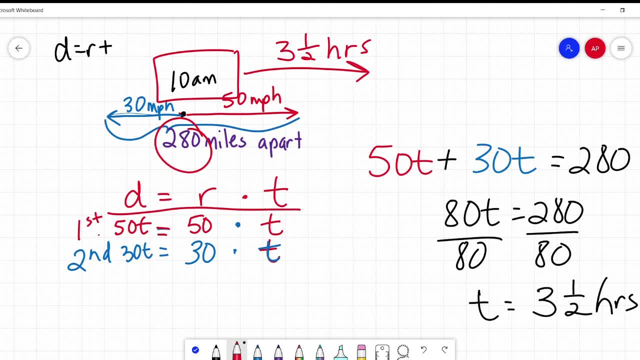 when you're dealing with time, just go like: okay, one hour to 11,, two hours to 12,, three hours to one. at 1: 30 PM, they will be 280 miles apart. Okay, Sorry, Sorry. Shame on me for not turning my. 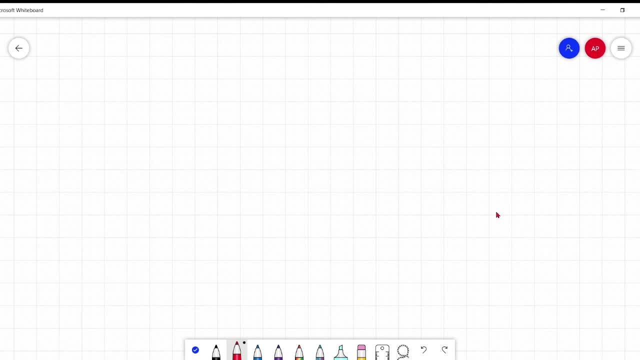 phone off. Sorry about that. Okay, So a second one right here. All right, Here's another one that they'll give you. They will give you, alright. so now we have two cars that are starting from the same point: The first car, the previous one- remember they started at the same time- This one, they're. 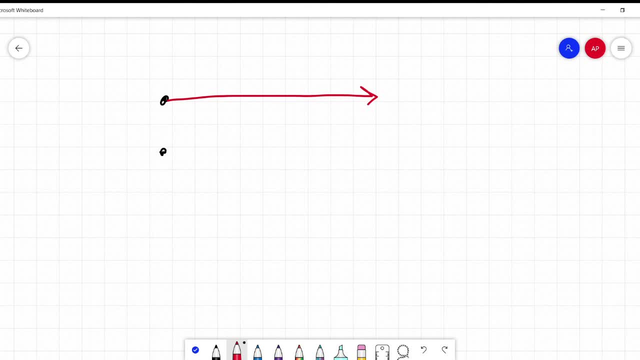 starting at the same point but they're leaving at different times. So I'm going to say the first one starts at 8 am, okay, and leaves going 50 miles per hour. The second car starts one hour later and is trying to catch up and it's going 65 miles per hour. At what time does he catch up? 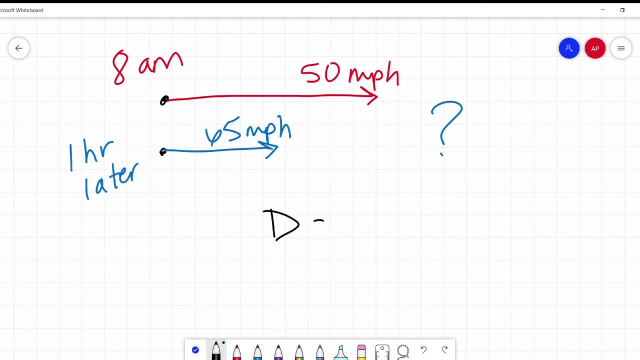 Okay, same sort of thing. Distance equals rate. times time. I'm going to fill in what I know. My first one: do I know the rate? Yes, I do. The rate is 50 miles per hour. Rate of my second one. 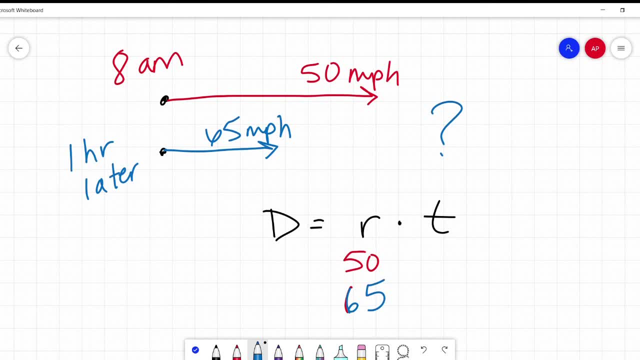 what is it? It is in blue: 65 miles per hour. Now the time for these two is not the same. I'm going to use T? T to represent the time that the first car, the 50 mile per hour car, the time that it drove. 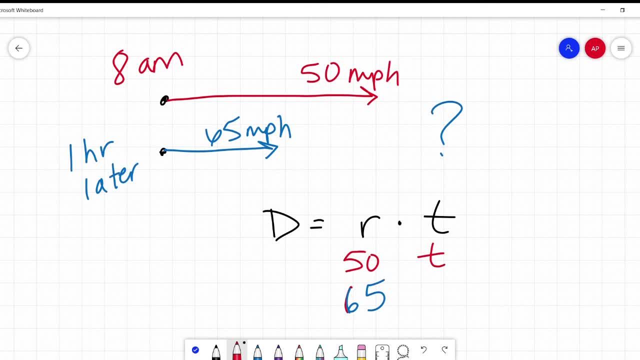 Now assuming again: they don't stop. they don't take potty breaks, they don't stop for any reason. The 50 mile per hour car drove T hours. How many hours does the 65 mile per hour car drive before it catches up? T minus T minus one. 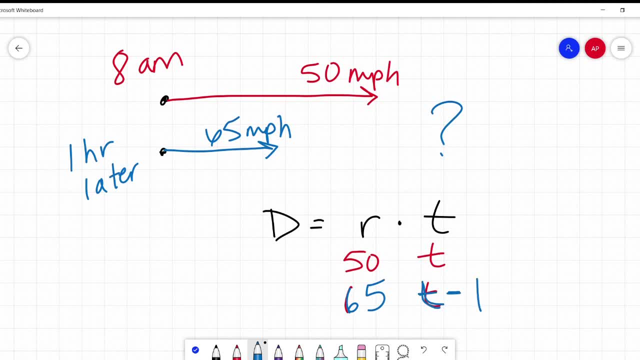 It leaves one hour later, So their driving time is one hour less. Same thing. I'm going to multiply 50 times T is 50T. 65 times T minus one. You do it like. you distribute it: 65 times T is 65T. 65 times negative one. 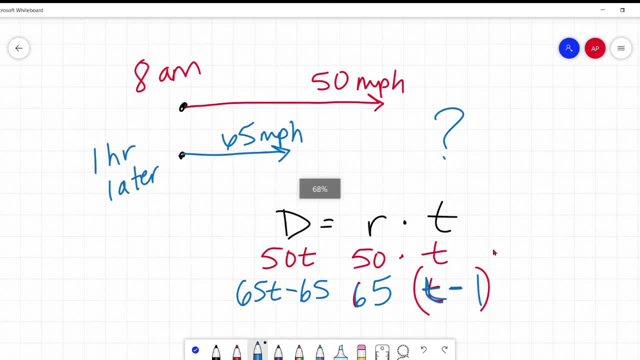 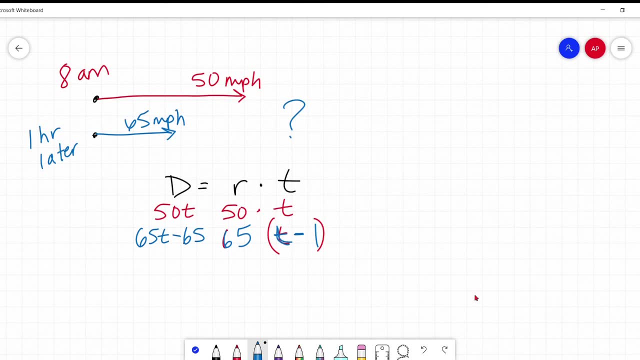 negative 65. Now, by the time they catch up because they're driving in the same direction, they're both driving the same distance. They, they come at that same point, They come and meet each other at that same point, So we can set the distances equal to each other. That's the difference. on this one We're not adding. 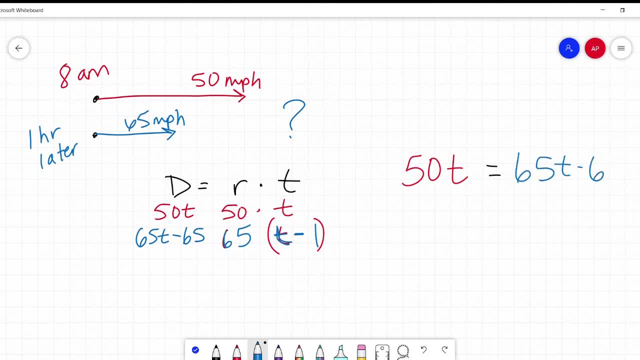 to anything. We're setting them equal to each other because they're driving the same distance. Okay, So I'm going to solve this. I'm going to subtract 65T from both sides and I get negative. 15T equals negative 65.. 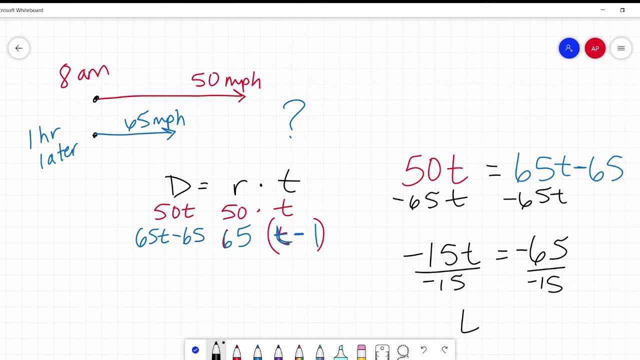 I divide both sides by negative, 15 t equals four and one third. if I'm talking about time, one third of an hour. so it's four hours and 20 minutes. if they leave- see back up here- they leave at 8 am. four hours and 20 minutes. they're going to meet at 12: 20 pm and didn't register there. 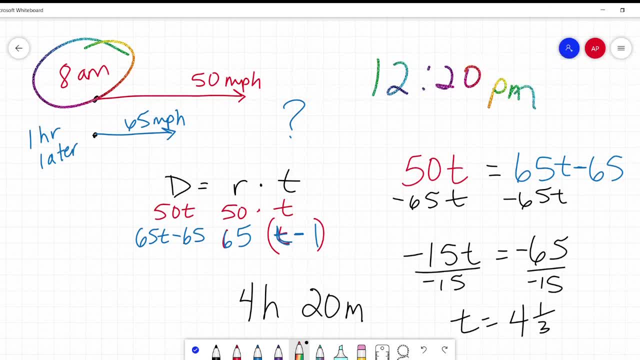 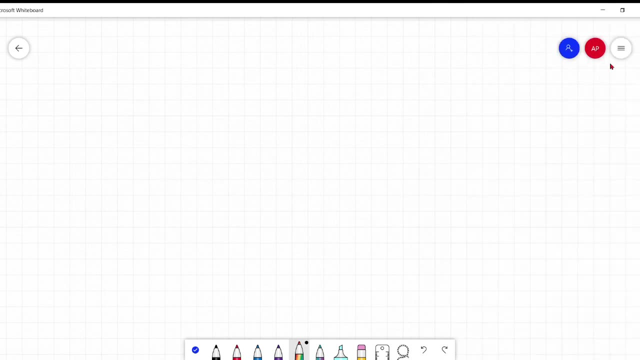 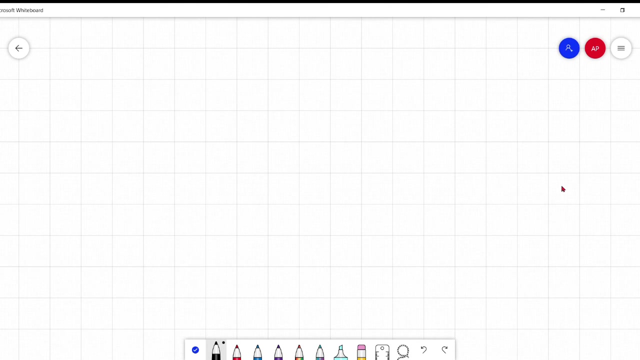 it's not registering. there we go. finally, it doesn't like my rainbow pen. sometimes, I don't know why, it has issues at 12: 20 pm. okay, here's another example for you. clear this off, all right. third example: okay, so our third problem is going to be a little different. just to show you, um. 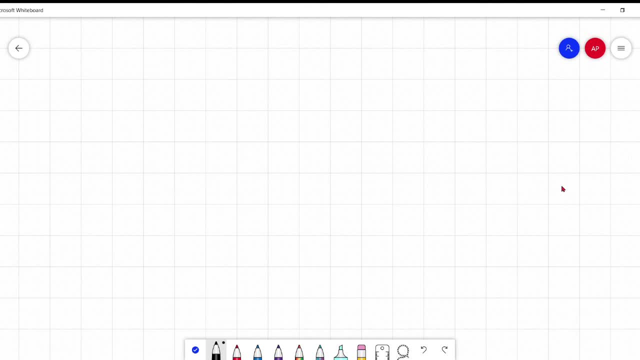 sometimes the, the variable they're asking for, the, the thing they're asking for can change um. let's say, I had two cars starting at two different cities and they're driving towards each other and the first one is going 45 miles per hour and our other one is going 55 miles, 55 miles per hour. 55 miles per hour. 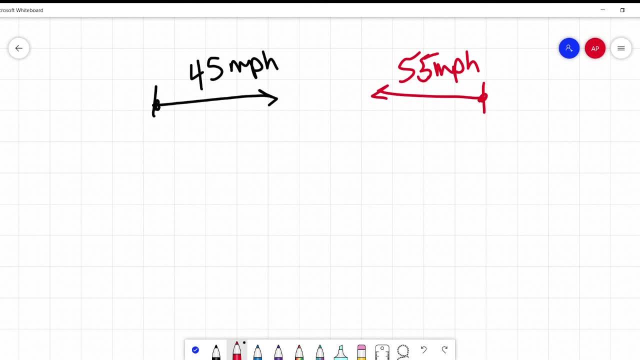 okay, so after two hours they pass each other because they're on a normal road, they don't have a collision, they just start going along their merry way and they pass each other. and there's that point where they go past each other. it takes it two hours. how far apart are the two cities? well, we can still use. 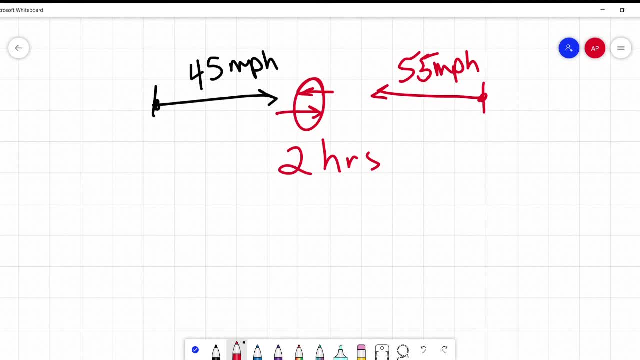 our same distance equals rate times time. um, some of you who you know, really kind of like, okay, I'm getting this, I'm getting this. you may think, well, I don't need to write this out, but you have to remember it's an issue that doesn't keep you together. it's also a case of missing data and 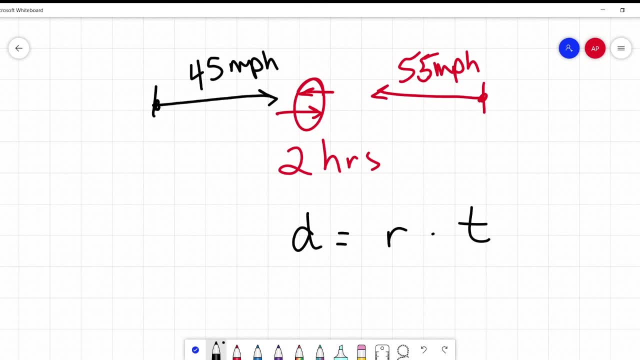 you just kind of need to thank God, and another thing that you have to protect yourself from is you have to actually do out there and keep track of that. so this one just gets newer, and you have to wait till you get to that point. leave your imagination and let your brain lay scissors shut before you. 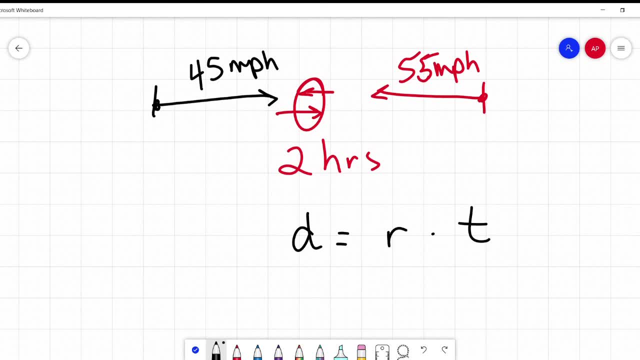 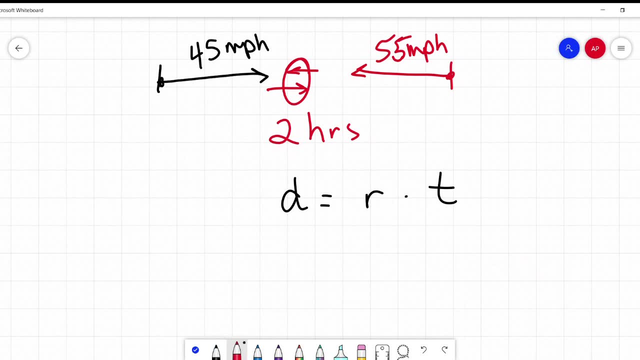 You may think: well, I don't need to write this out, It's still a good habit to get into. You're less likely to make mistakes, Okay, so in any event, we're just going to write everything out. So our rate for the first car is 45 miles per hour. 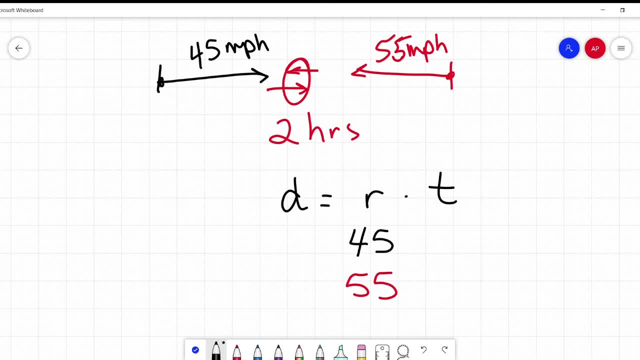 The rate for our second is 55. The time is two hours for both of them. I've had some students say, well, that doesn't make sense. This one's going at that speed and they're going these different things. It's two hours at the same time. 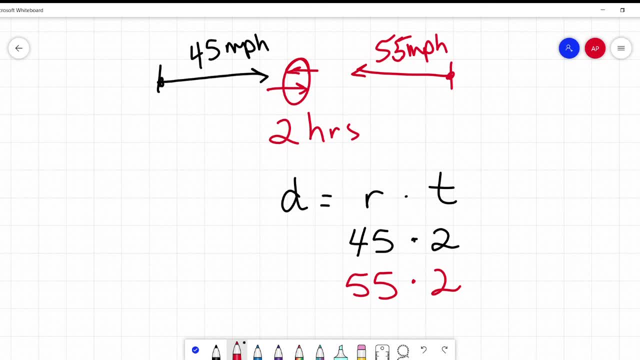 I said yes, it is because you know they both left at 10 am. I'll say: they both left at 10 am. They started driving towards each other. No one stopped for a bathroom, No one stopped for any reason. 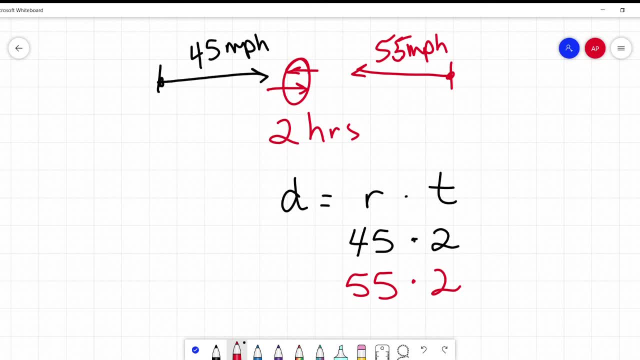 They just got in the cars and they drove and they passed each other at 12.. They've both been driving for two hours. They've gone to different distances but they've both driven for two hours. So I just multiply this together: 45 times two is 95.. 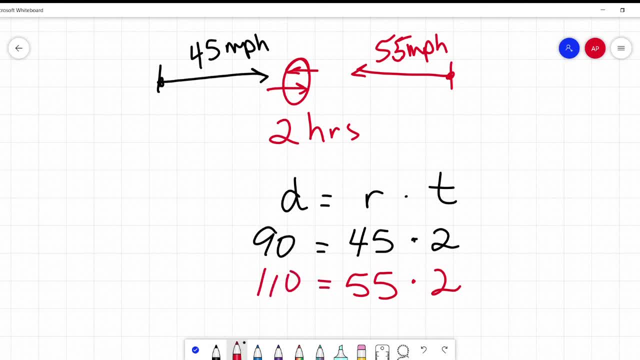 So 90 miles 55 times two is 110. And then all I have to do is add those together: 90 plus 110.. The cities are 200 miles apart. Okay, Now, this still would have worked if it had been similar to some of those other problems we did. 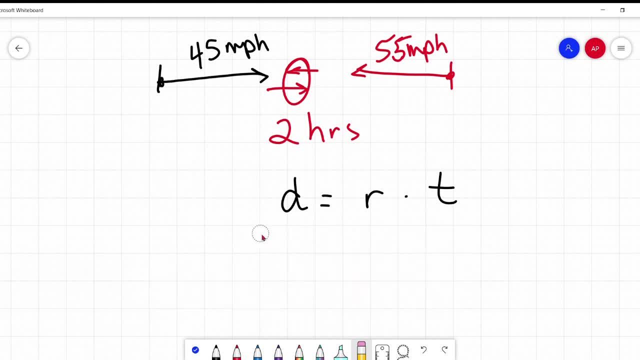 where they don't tell us the time and instead they tell us the distance. So let's say, they say: These cities are, Come on, There it goes. These cities are 200 miles apart. How long does it take before the cars pass each other? 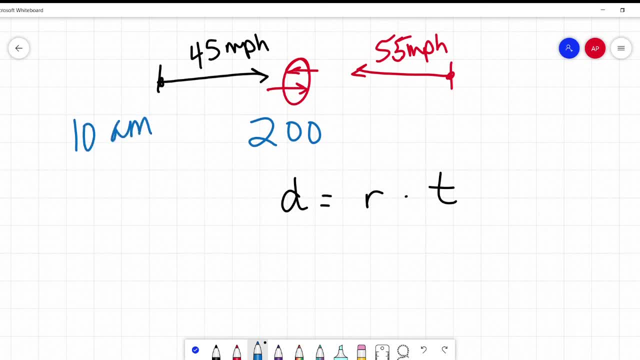 They might even say they leave the cities at 10 am. precisely At what time do they pass each other? Okay, Same thing. The one thing I want to reiterate with this: Some people, they go oh distance. 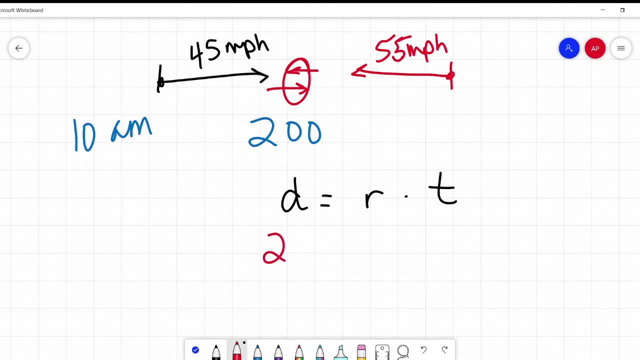 It's 200 miles And they just write that down And that will throw you off. You'll get it wrong. Don't do that, Because they're not traveling 200 miles, They're each traveling a portion of the 200 miles. 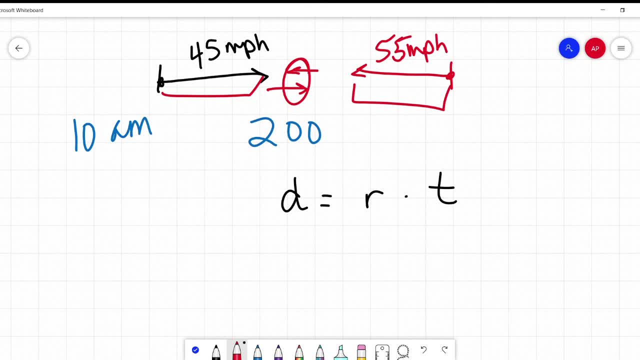 Together it's 200 miles, but not individually. So if I start writing 200 for both of them, No, no, no, We don't want to do that. Okay, So our rates are 45 and 55. Okay. 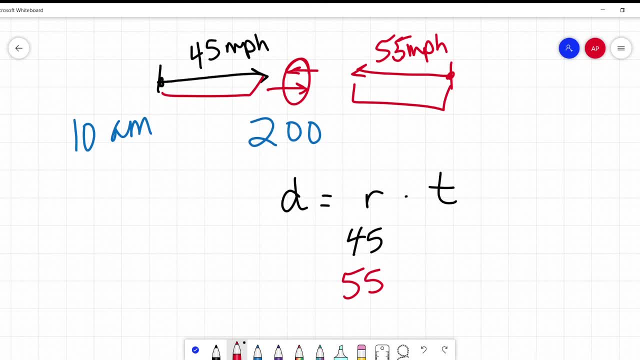 The time. we don't know, That's our unknown, But we know it's the same for both of them. So it's just T for both of them. Okay, And same sort of thing. We're going to say: rate times: time 45 times T equals the distance 45T. 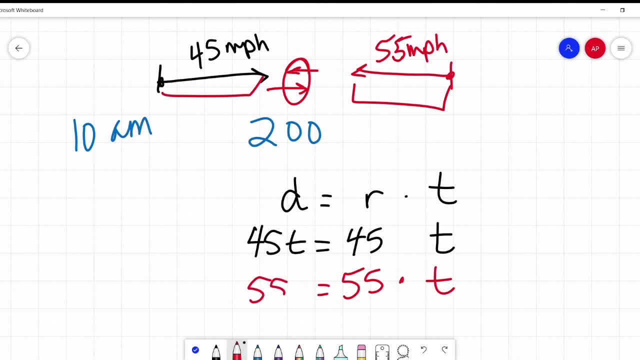 This one rate times time. 55 times T is the distance: 55T. Together these distances equal 200.. Okay So 45T plus 55T is 100T. That equals 200.. And I divide both sides by 100. 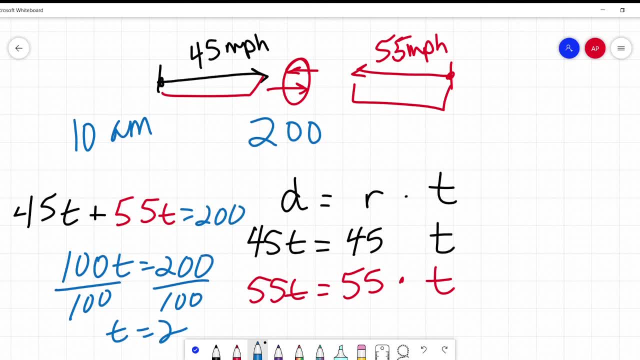 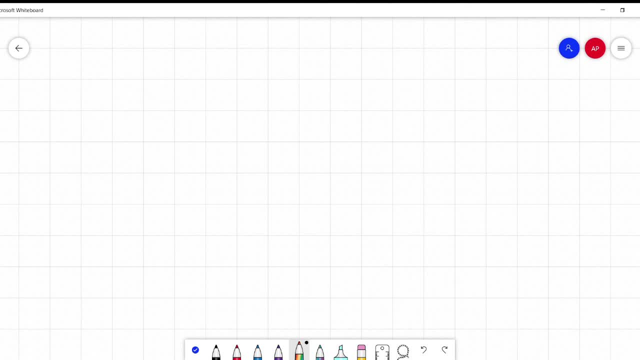 And T equals to two hours. They leave at 10 am, They pass each other at noon. Okay, So I know I mentioned a bonus problem, but this has gone on. I think I'm at like about 15 minutes. This is. it's going to be too long. 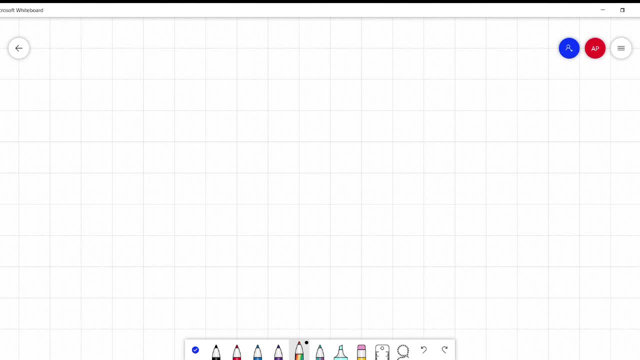 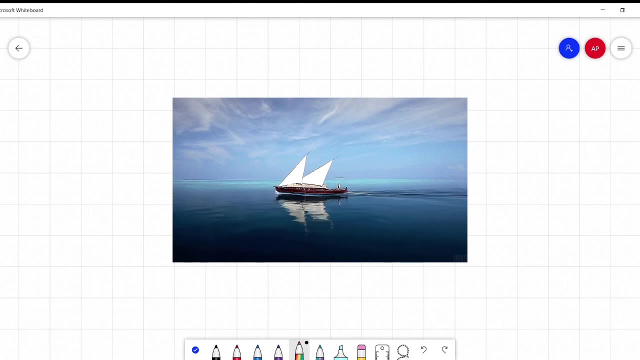 So I'm going to split this up. This is a part one. Part two, the bonus problem. That's the one you're going to go to if you are dealing with a distance rate time problem. that has things like: I have a boat in a current and the current is pushing it faster or slowing it down in opposite directions. 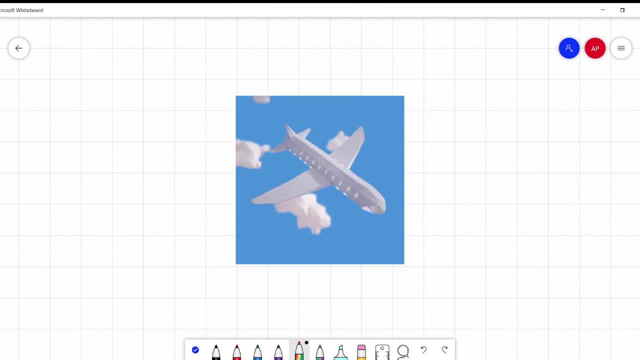 Or if you have a plane that, okay, in one direction it's going with the wind, other it's going against the wind. A problem that includes that type of thing is in the second part. Okay, So link to that is in the description below. 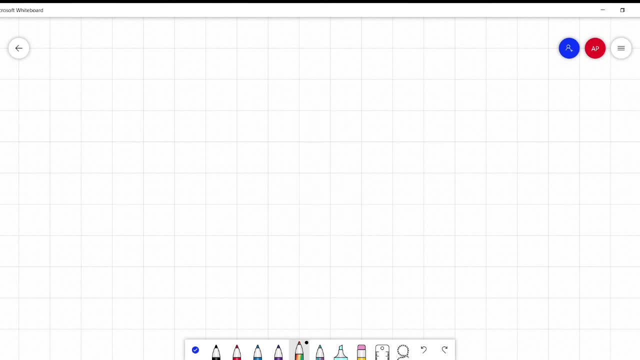 So please click on that If that's the type of distance rate problem you have, because that takes some explanation. that in itself is like 10 to 15 minutes to go through and thoroughly explain everything that's going on with that. All right.